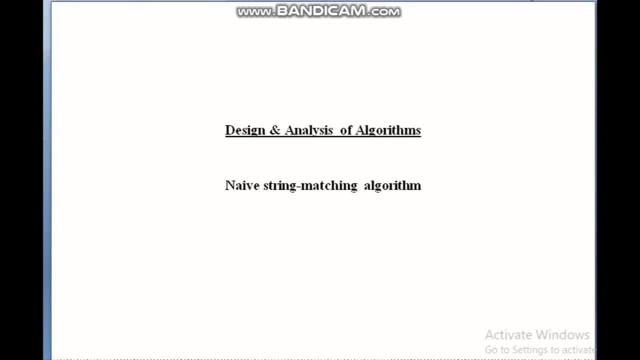 Today we are going to discuss very basic concept of string matching algorithm. that is the name: string matching algorithm. What is string matching algorithm? String matching algorithm is basically an algorithm that try to find a place where one or more patterns are found within a larger string. 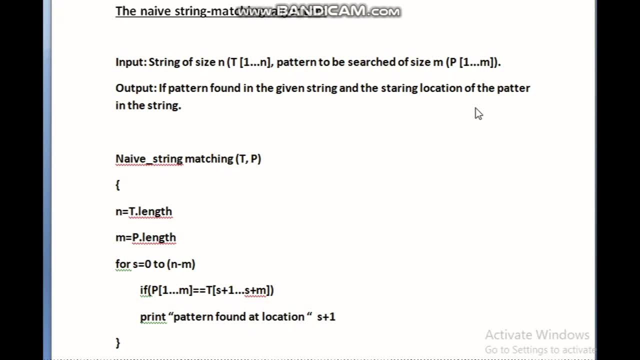 Let's look at the algorithm Here. the inputs are string of size n, that is, p of 1 to n. pattern to be searched of size n that is p of 1 to n. Output is pattern found in the given string and starting locations of the pattern in the string. 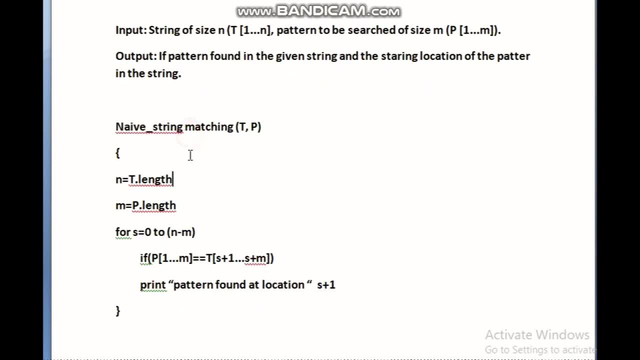 And the data code for the algorithm is: We pass two array, t and b, And in n we put length of string t and we put length of the pattern in n And we start a whole loop to check whether this pattern is present in the strings or not. 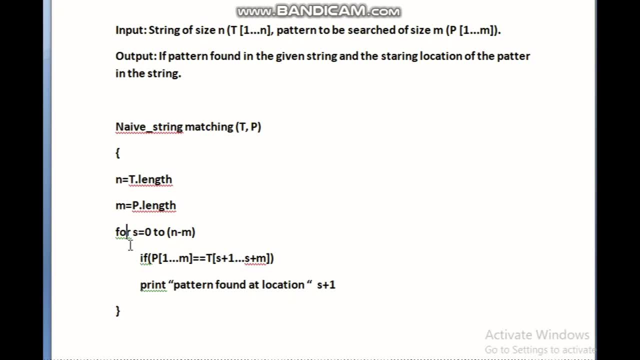 So you see How much time we run. We run s equal to 0 to n minus n, Because if you run more than that time, then the size will be. There will be no element to search for, every element. That's why we will run from 0 to n minus n time. 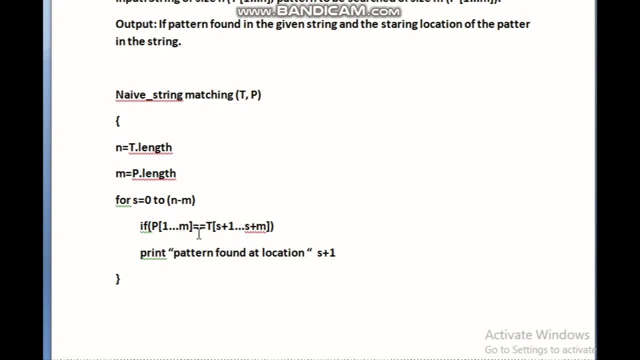 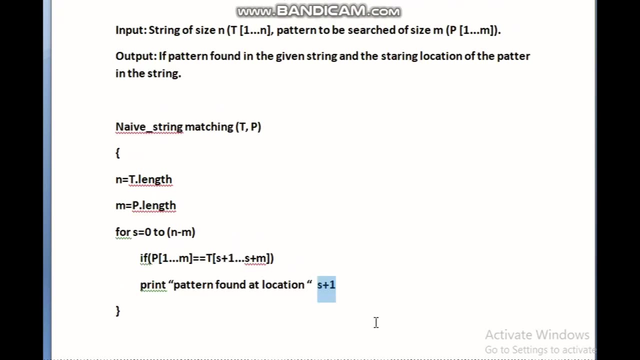 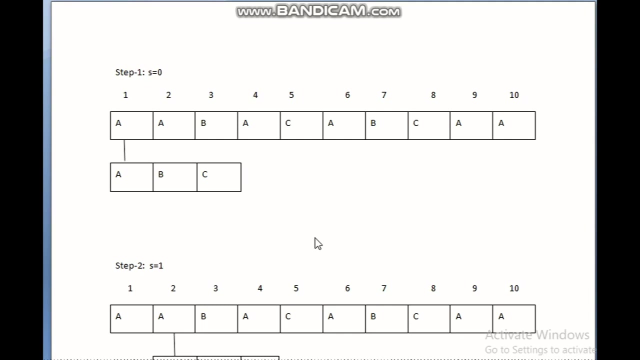 Each element of pattern will be compared to the strings. If it is true, Then we change the location. That is s plus 1.. Let's see an example. Suppose we have a string of length 10.. That is a, a, b, a, c, a, a, c, a a a. 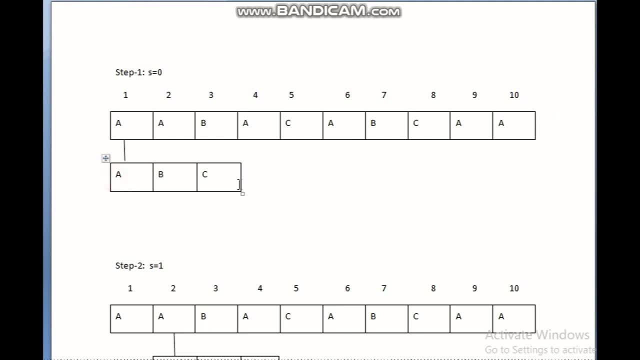 And we have pattern a, b, c, We have to check whether this pattern is present in the string. Is it present in the string or not, As in this algorithm, Starting from 0, s equal to 0 to n minus 1.. 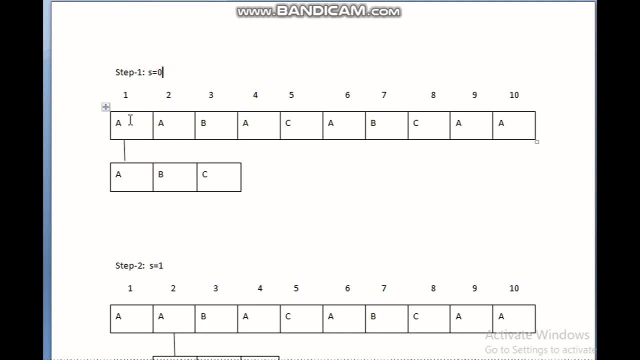 That is, we start from here- s equal to 0.. Pattern p of 1,, 2,, 3 will be compared with strings s plus 1,, s plus 2,, s plus 3.. That is s equal to 0.. 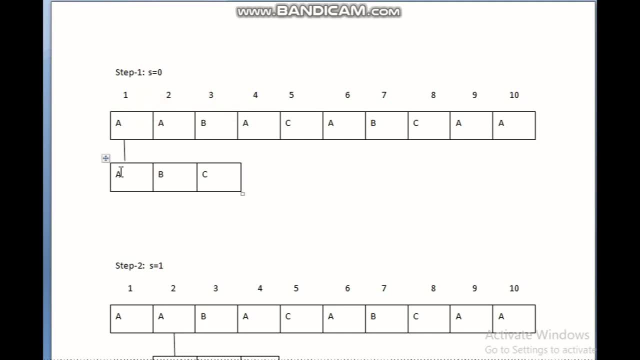 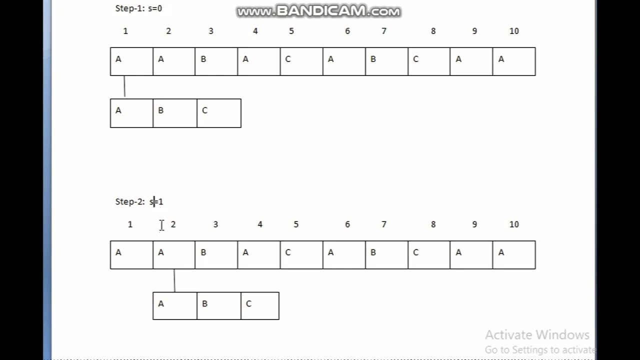 1,, 2, 3.. This string element will be compared to this string. Here first is matched, But second here is unmatched. Here also there is unmatched, So it will move to next. a Here s will be infinite and s equal to 1.. 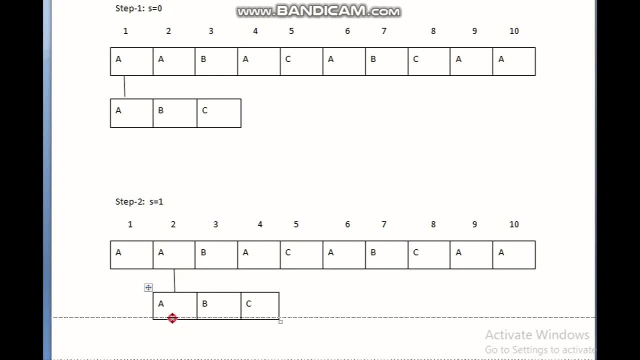 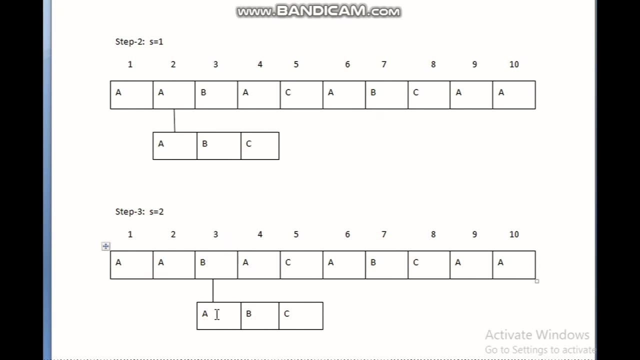 So second element will be compared: These two are matched. So there is, there is matched, These two unmatched, So it will move to next. a Here s equal to 2.. So the pattern a, b, c will be compared with b a c. 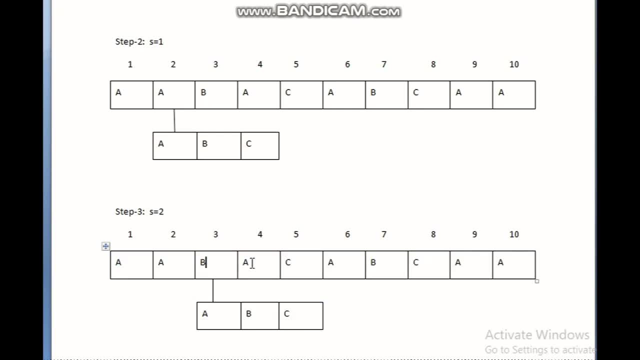 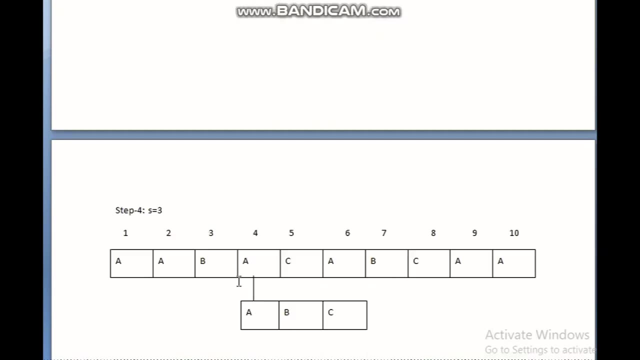 Here. this is unmatched, This is unmatched, This no matter. If single element is unmatched, then it means the pattern is not present. So move to next a. So move to next s, s equal to 3.. That means s of c plus 1, c plus 2, c plus 3.. 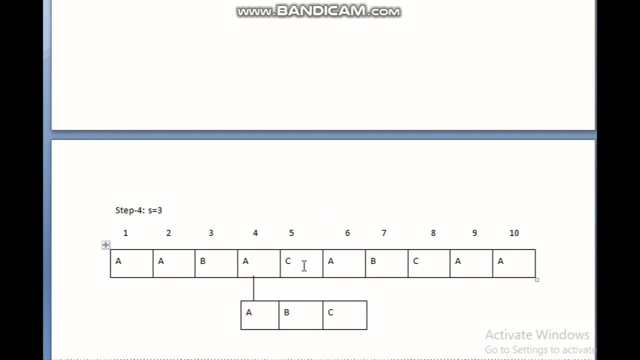 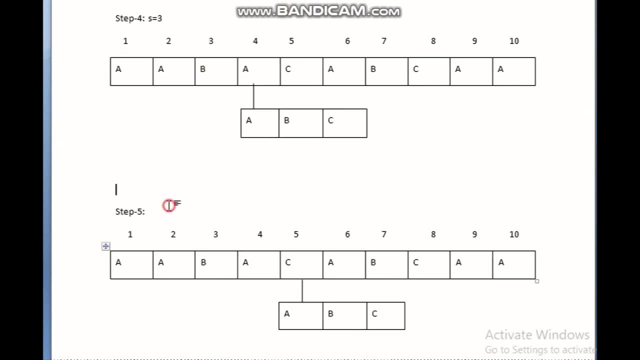 So a will be compared to this: unmatched, There is unmatched, There is unmatched, So it will move to next step. Here s become 4.. So, starting from s plus 5. It will be compared to: there is unmatched, There is unmatched. 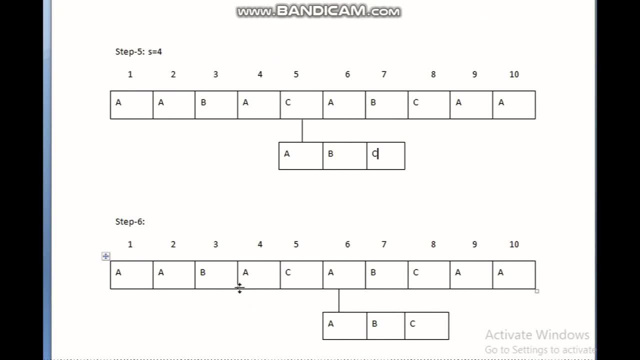 Unmatched, So it will move to next step. Step 6 here s equal to 5.. So pattern t of 1,, 2, c will be compared to it. Text 5 plus 1 means 6,, 7, 8.. 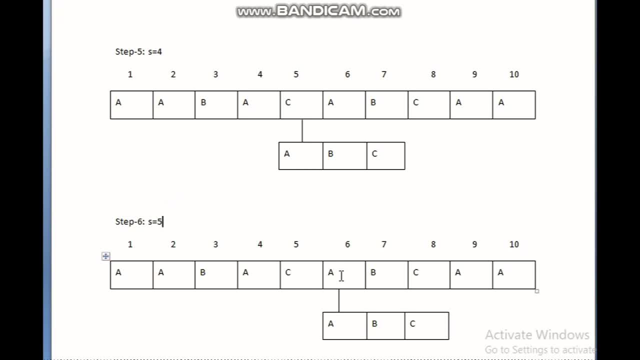 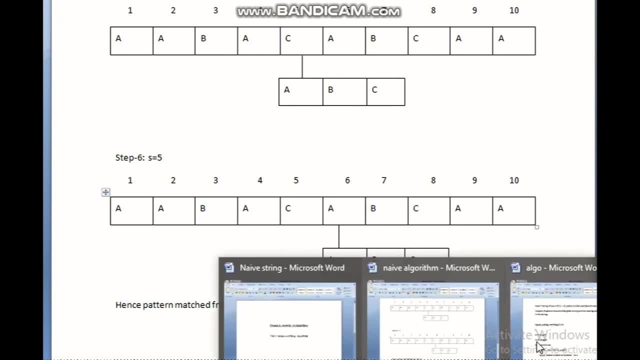 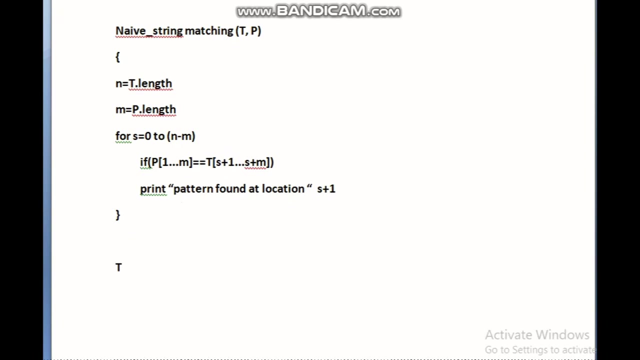 Oh, there is unmatched. Each element of the text is matched with each element of the pattern. Hence the pattern matched from location 6.. This location will be returned to the new page. Page, Page, is it? Page is all Now. analyze the time complexity for the algorithm. 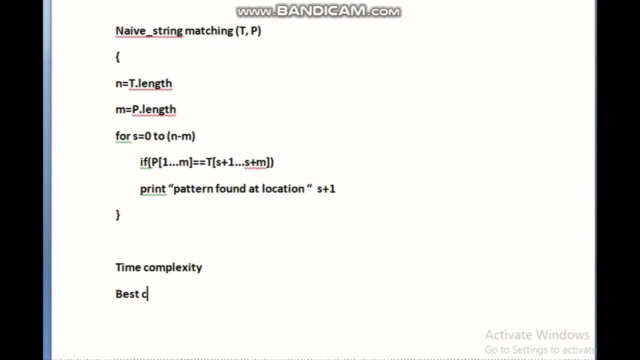 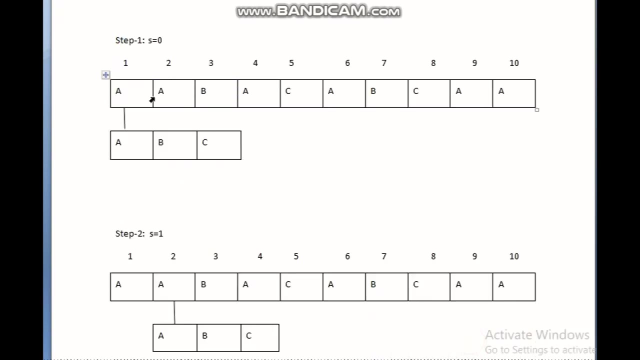 In best case time complexity when the algorithm takes minimum time. if the pattern found at the beginning of the streams, then it will take minimum time, then the time complexity will be perfect For best case time complexity when the algorithm takes minimum time, then it will take minimum. 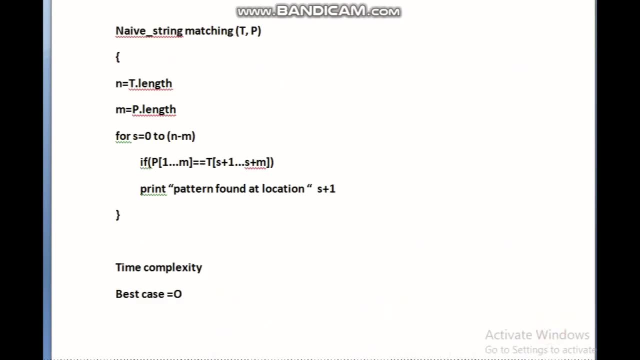 time, then the time complexity will be perfect. In order of M. the N elements of the patterns need to be set to M elements of the streams. if the length of the pattern is one, then the удders is one, And also the sum and the間 value of strata, say, is also same. 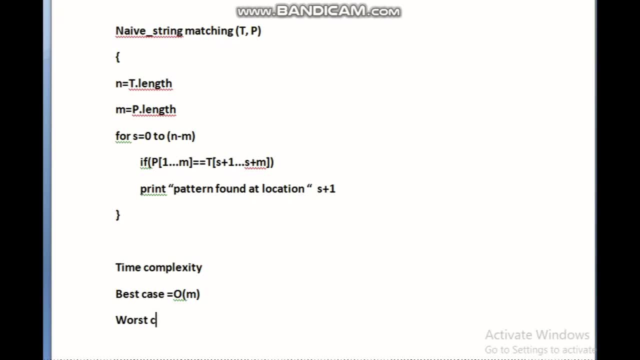 Ok, fine, Next is the time. complexity will be. see how much time the loop will executed: 0 to n-n. so if the patterns appear at the rightmost side of the string or it does not present at all in the string, then it will take the maximum value. 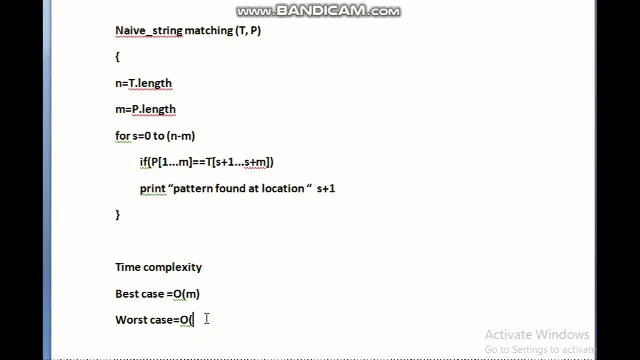 Therefore the complexity for worst case will be order of n-n. say, the loop will started from 0, that is, n-n plus 1 into n, because each time m element of pattern need to be checked with n element of the string. Thank you.